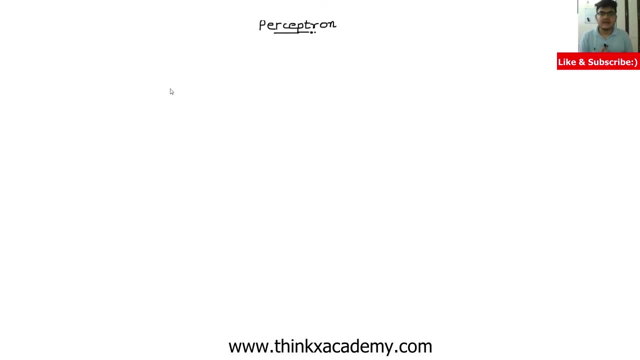 Hi thinkers, welcome to ThinkX Academy. In this machine learning playlist, we have already discussed artificial neural networks. In this tutorial, we are going to cover perceptron, which is basically a simplistic version of the neural networks that we have studied. So what is a perceptron? A perceptron is a supervised learning algorithm. 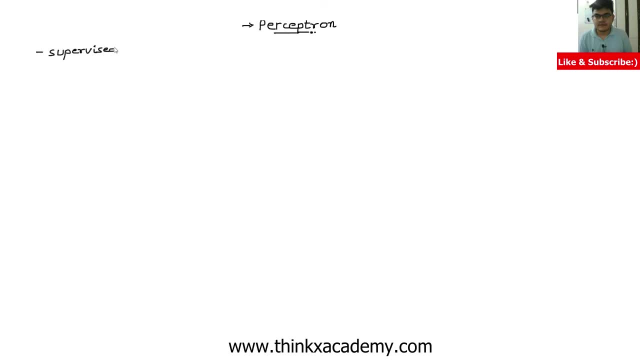 So it is a supervised learning algorithm, which basically means that we are actually given a data set in the form of features and we also have a mapping, So we will have a data set, something like this. We have already discussed this data set in the previous tutorials of linear. 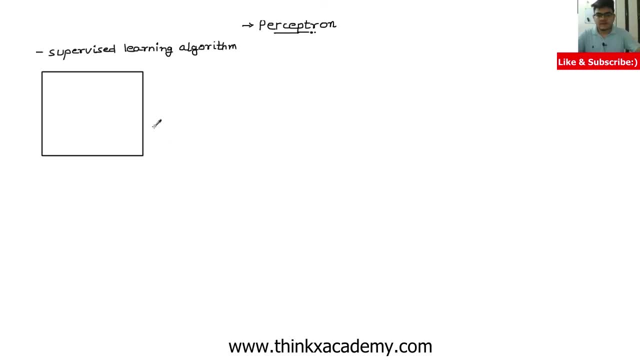 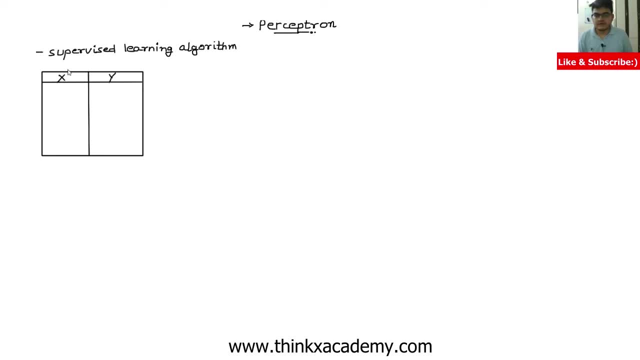 has a mapping to y. So for every value of x I have a mapping to y. So perceptron basically is a learning algorithm and it is a supervised learning algorithm because we have a supervision of some output mapping. So the second thing about perceptron is that we will use 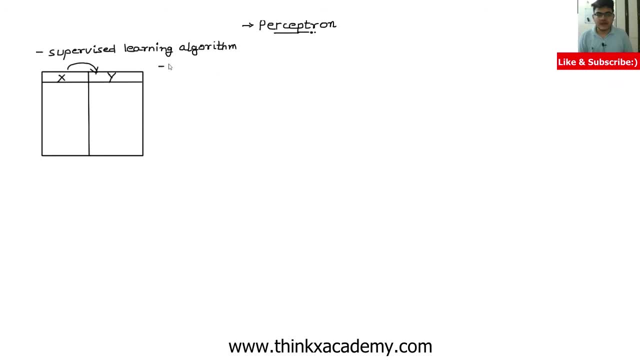 perceptron to do the classification and, more importantly, a binary classification. So basically, perceptrons are binary classifiers, which means that they convert the data into two classes. right, So first we will train the perceptron learning algorithm with the given. 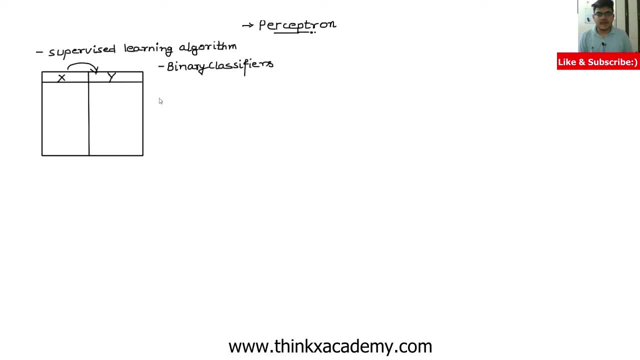 data set, with the given inputs and output mappings, And then we will test it with some samples. So we will train the perceptron learning algorithm with the given data set, with the given input mappings, And then we will test it with some samples. So we will train the. 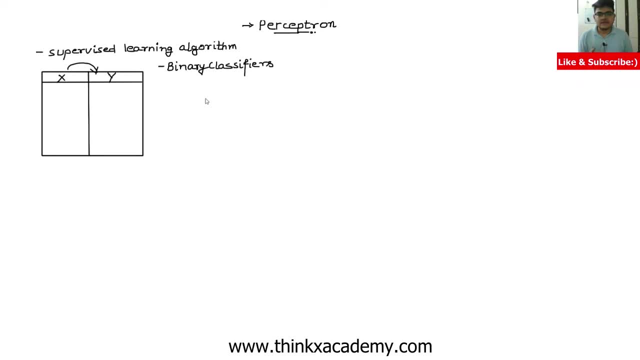 perceptron learning algorithm with the given data set, with the given inputs and output mappings, data as we used to do it in linear regression, and all the learning algorithms that we have studied. So perceptron looks similar to a neural network, So I'm going to now show you a basic. 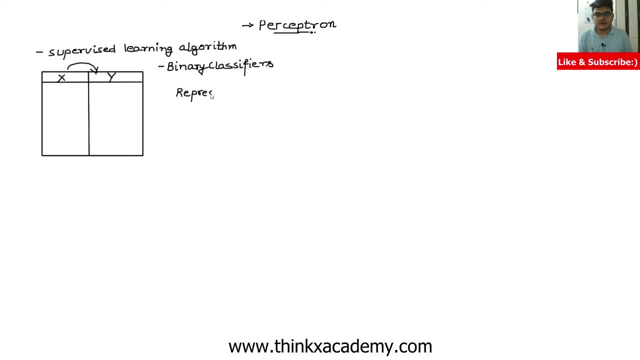 representation of a perceptron so that you will be able to understand how it is similar to the neural networks. It is just simpler than the neural network. So in neural network we know that we have the input features, So we have the input features. we have the input features, we have the 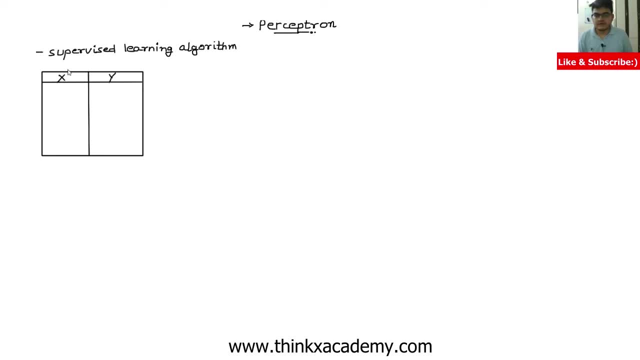 has a mapping to y. So for every value of x I have a mapping to y. So perceptron basically is a learning algorithm and it is a supervised learning algorithm because we have a supervision of some output mapping. So the second thing about perceptron is that we will use 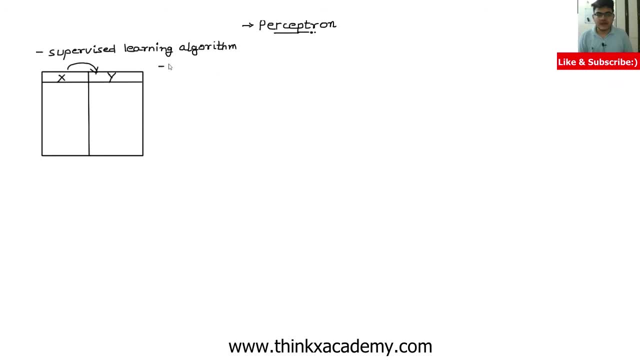 perceptron to do the classification and, more importantly, a binary classification. So basically, perceptrons are binary classifiers, which means that they convert the data into two classes. right, So first we will train the perceptron learning algorithm with the given. 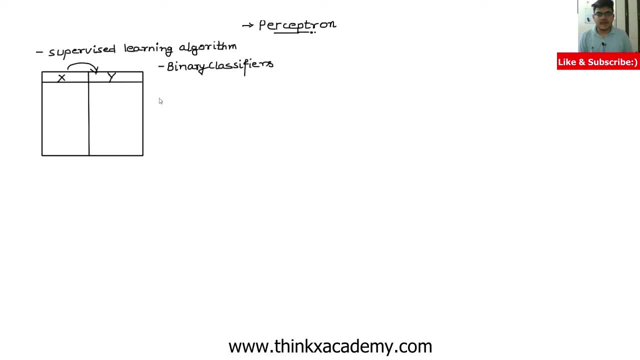 data set, with the given inputs and output mappings, And then we will test it with some samples. So we will train the perceptron learning algorithm with the given data set, with the given input mappings, And then we will test it with some samples. So we will train the. 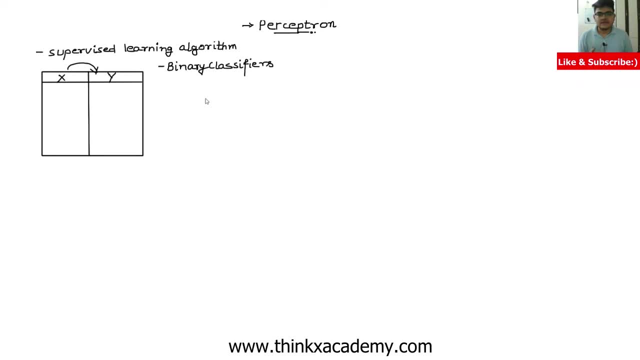 perceptron learning algorithm with the given data set, with the given inputs and output mappings, data as we used to do it in linear regression, and all the learning algorithms that we have studied. So perceptron looks similar to a neural network, So I'm going to now show you a basic. 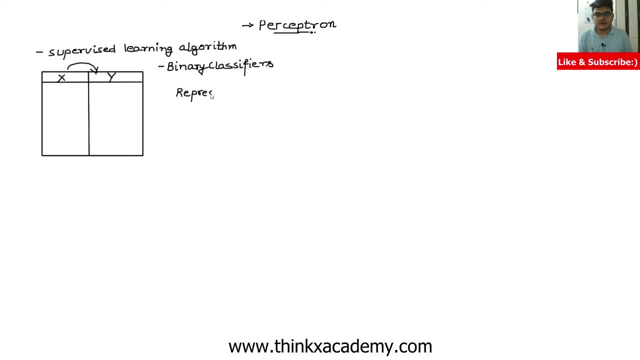 representation of a perceptron so that you will be able to understand how it is similar to the neural networks. It is just simpler than the neural network. So in neural network we know that we have the input features, So we have the input features. we have the input features, we have the 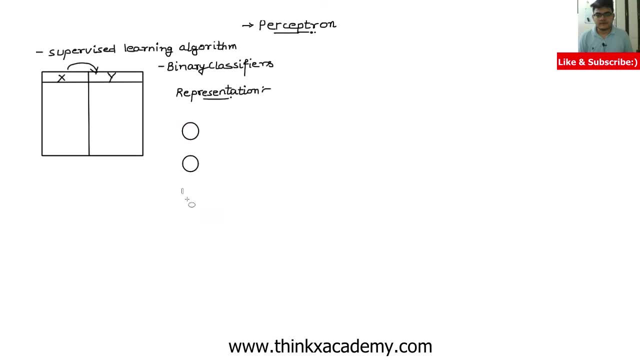 input layer, right? So let's say, we have these input features, which is, let's say, x1,, x2, and x3.. So we have an input layer here. You can see that Now. what we do is we try to make a channel. 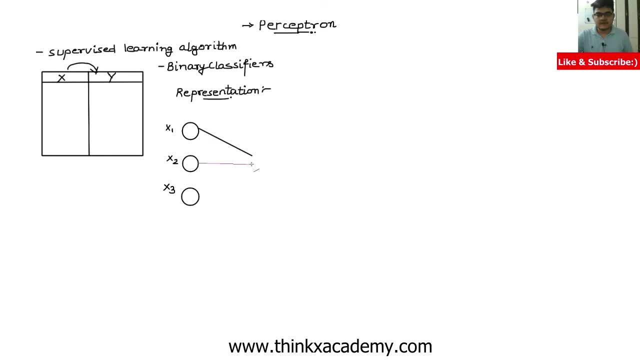 through all of these inputs And basically, these are the weighted channels. This means that these channels actually has some weight which is assigned as weight one, weight two and weight three. Now, if we have n number of features, we will have x n number of features And similarly. 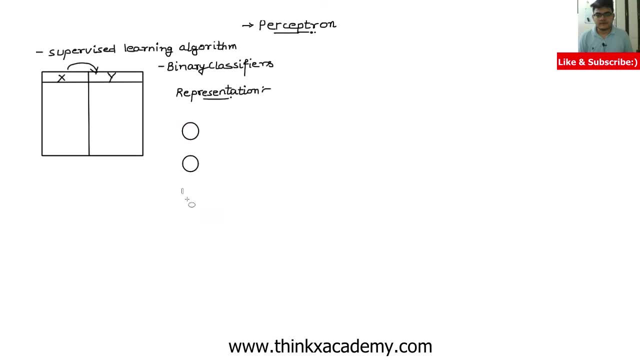 input layer, right? So let's say, we have these input features, which is, let's say, x1,, x2, and x3.. So we have an input layer here. You can see that Now. what we do is we try to make a channel. 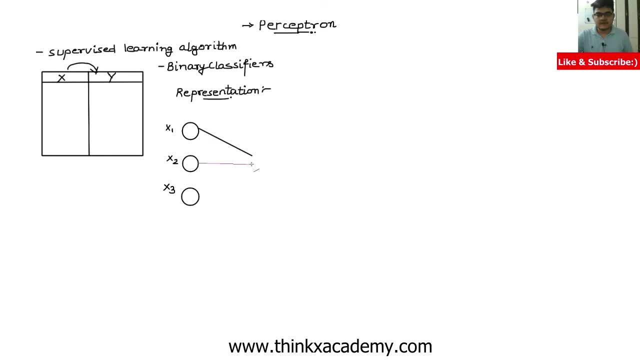 through all of these inputs And basically, these are the weighted channels. This means that these channels actually has some weight which is assigned as weight one, weight two and weight three. Now, if we have n number of features, we will have x n number of features And similarly. 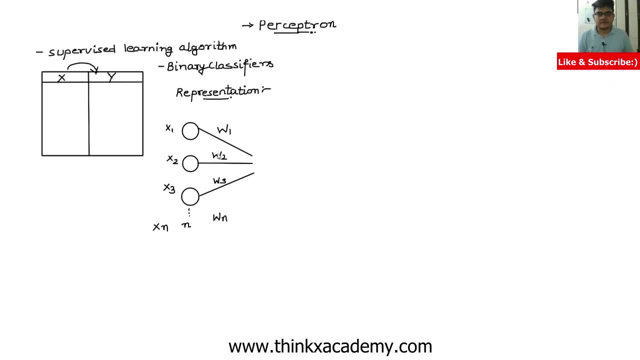 we will have w n weights right. So what we do in a perceptron is that we actually try to make component here. let's make another component here. Here we will make a component which is basically a circuit which does this operation, which I'm going to write here: x1, w1, plus x2, w2.. 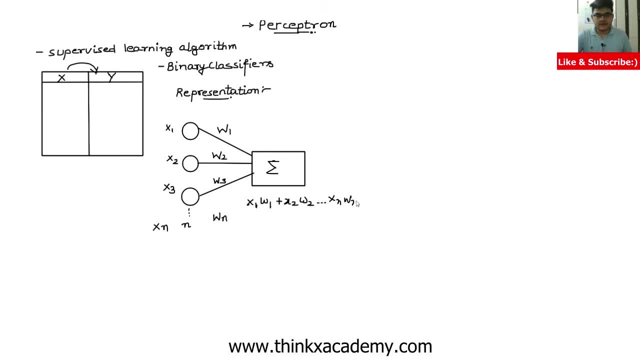 And it goes on till x, n, w, n, right, So this circuit is basically an adder circuit- Sometimes it is also known as an adder- And what it does is it multiplies the components of the input features with the weights and it adds all of them. One more thing is that we also add a bias. 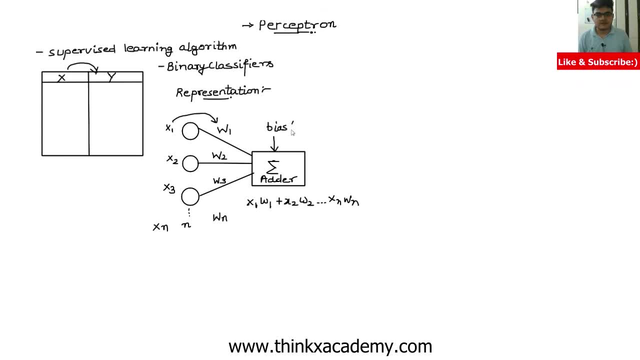 which is B right. A bias B is also added to each of these x1,, w1, right. So we also add a bias B to the output of this whole component. So when we pass through this component we will actually be. 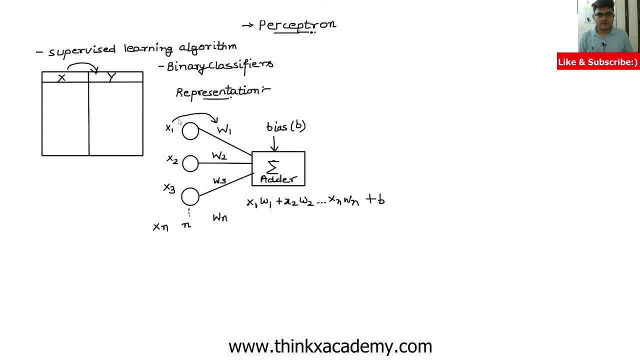 able to do the multiplication of all these features, And we will actually be able to do the multiplication of all these features and the weights, And we will also add a bias. And after calculating this result, let's say this is the result R- we pass it to the next component. 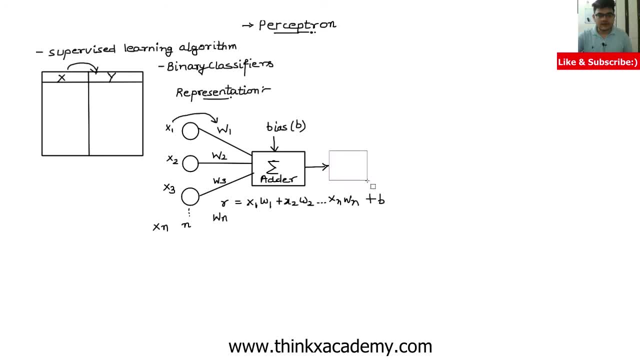 which is basically a activation function, And we have already studied that activation function is basically used to activate, which is basically a sigmoid function. So this is basically an activator And we will also add a bias And after calculating this result, let's say this is the result. 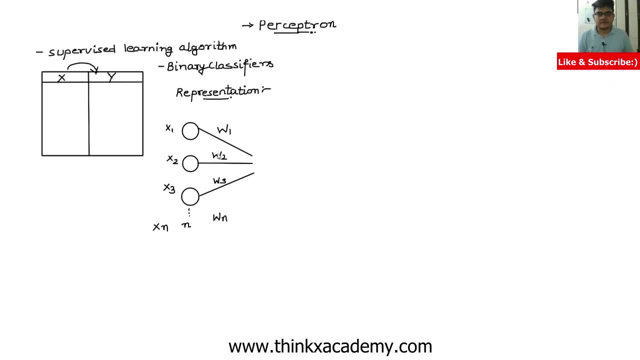 we will have w n weights right. So what we do in a perceptron is that we actually try to make component here. let's make another component here. Here we will make a component which is basically a circuit which does this operation, which I'm going to write here: x1, w1, plus x2, w2.. 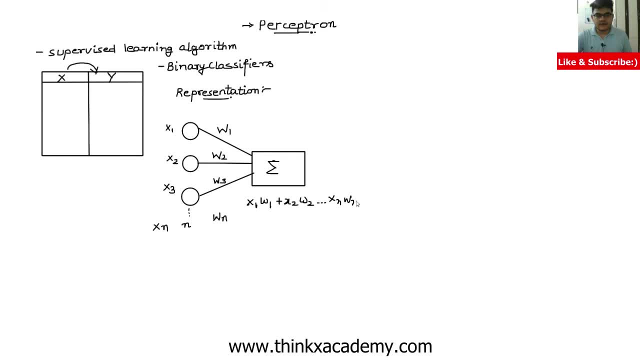 And it goes on till x, n, w, n, right, So this circuit is basically an adder circuit- Sometimes it is also known as an adder- And what it does is it multiplies the components of the output features with the weights and it adds all of them. One more thing is that we also 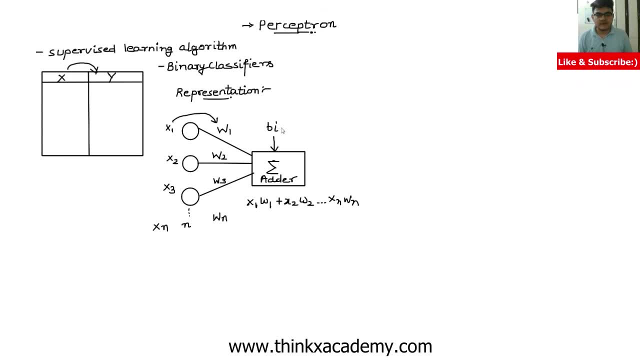 add a bias which is b right. Bias b is also added to each of these x1,, w1, right. So we also add a bias b to the output of this whole component. So when we pass through this component we will actually be able to do the multiplication. 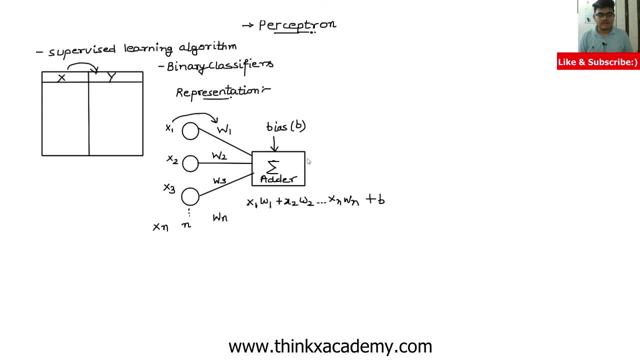 and the weights and we will also add a bias. and after calculating this result- let's say this is the result r- we pass it to the next component, which is basically a activation function, and we have already studied the activate. that activation function is basically used to activate. 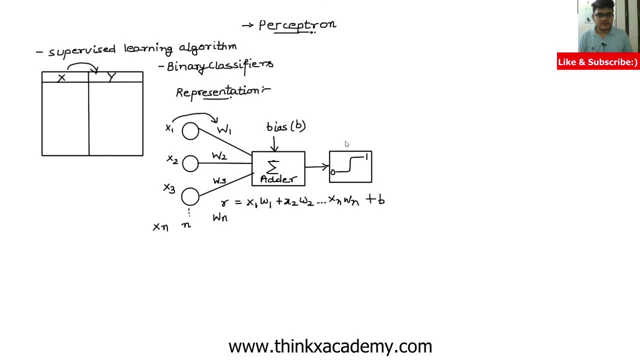 which is basically a sigmoid function. so this is basically an activator or a threshold. you can, you can even say that this is a threshold. so when the this input, which is this one- let me simplify this whole equation here we can actually simplify it as sigma goes from i equals to 1 till n. 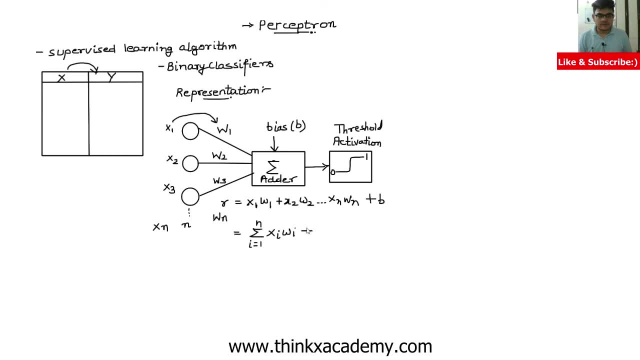 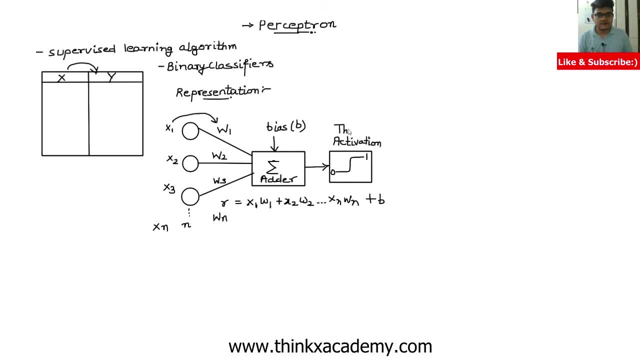 a threshold. you can even say that this is a threshold. So when this input, which is this one- let me simplify this whole equation here- We can actually simplify it as sigma goes from i equals to 1 till n, xi, wi plus b. Now let's say: these inputs are some. 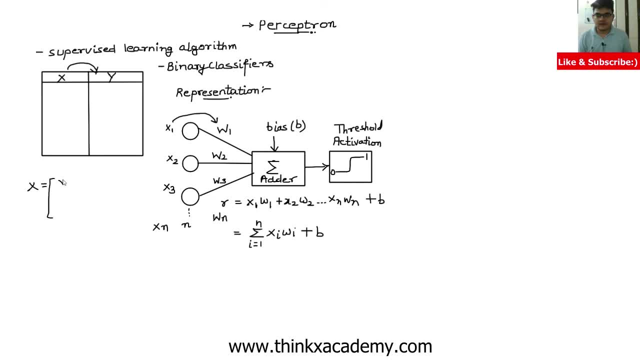 inside some vector x. So I will create a vector like this with all the inputs, And let's say we have another vector w which contains all the weights w1, w2 till wn, right, So we have these two vectors And basically this operation here, which you can see here, is actually just the scalar. 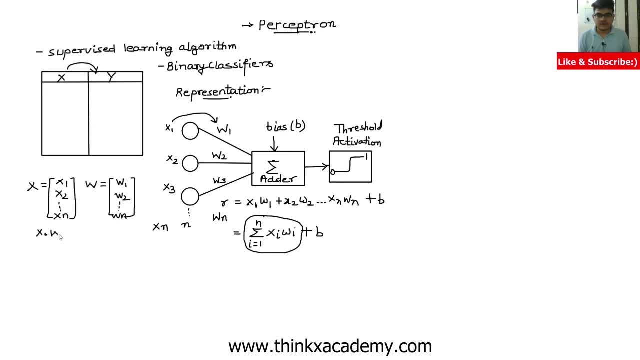 product of x and w. So x dot w will give me the scalar product which basically is multiply x1 with w1,, x2 with w2.. And similarly, we are going to add them up and we will get this, So we can actually write it as x dot w plus b. 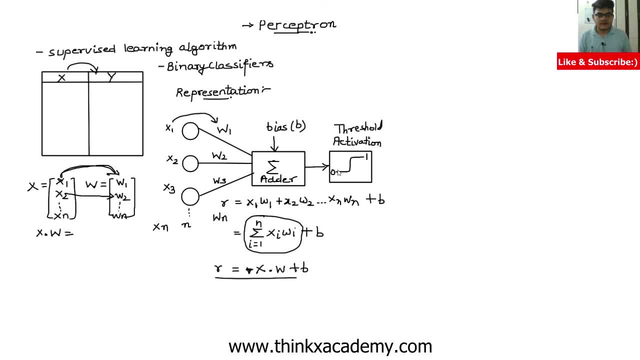 right. So this is the final result And we pass it to the threshold function. And what this threshold function does is that it actually classifies. it gives a value either as 0 or 1.. So if the value of x dot w plus b, which is the bias, 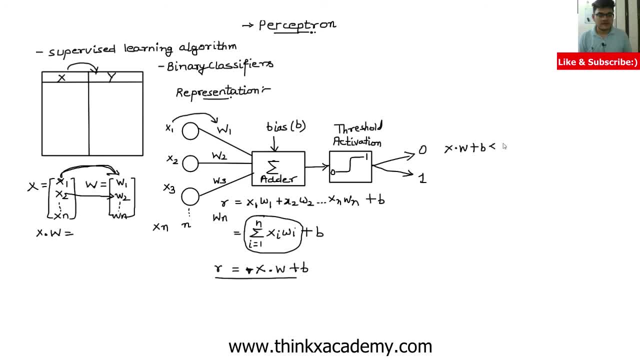 if this value is actually lesser than 0,, it will give a 0. And if this value is greater than 0, this will give me 1, right, So activation function. what it does is it classifies into whatever input you will give here. 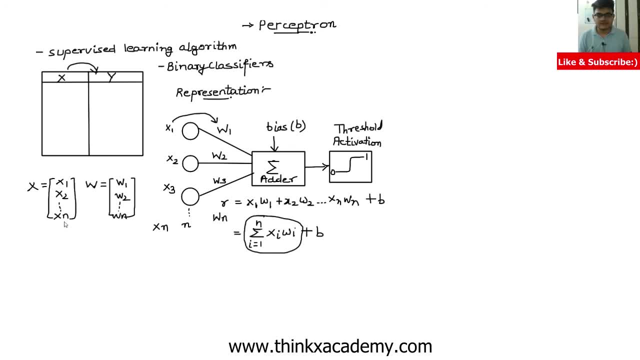 this operation here, which you can see here, is actually just the scalar product of x and y, and this is the scalar product of x and y, and this is the scalar product of x and y, x and w. so x dot w will give me the scalar product, which basically is multiply x1 with w1. 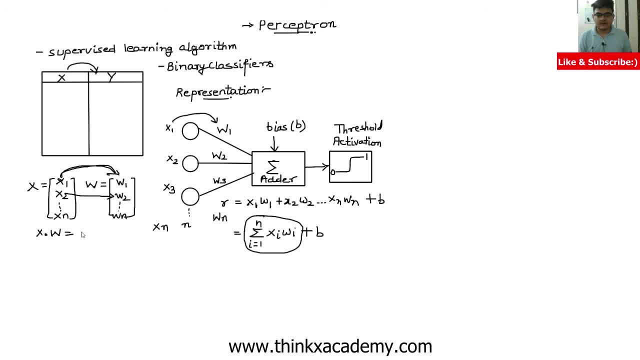 x2 with w2 and similarly. we are going to add them up and we will get this so we can actually write it as x, dot, w plus b, right? so this is the final result and we pass it to the threshold function, and what this threshold function does is that it actually classifies, it gives a value either as 0. 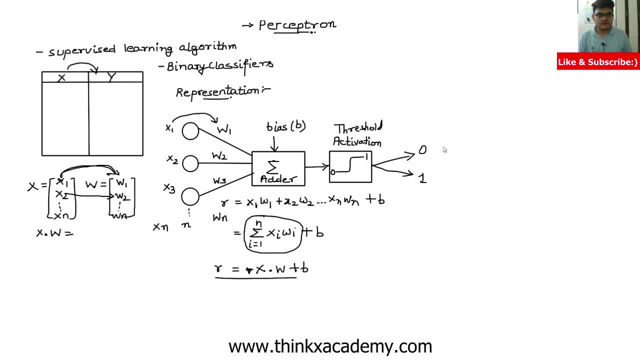 or 1. so if the value of x dot w plus b, which is the bias, if this value is actually lesser than 0, it will give a 0, and if this value is greater than 0, this will give me 1 right. So 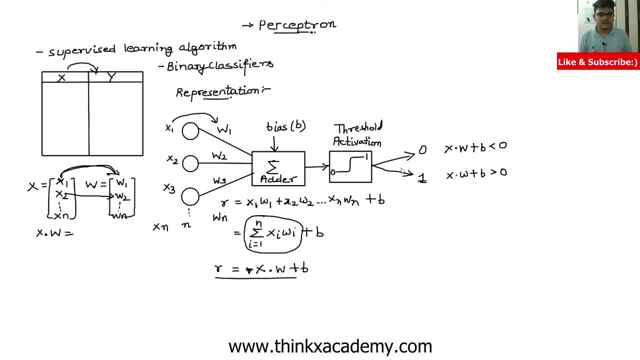 activation function. what it does is it classifies into whatever input you will give here it, since it is a sigmoid function, it will give an output as 0 or a 1, so it will classify it like this. So basically, a sigmoid function is this: f of x 1 upon 1 plus e raised to the power. 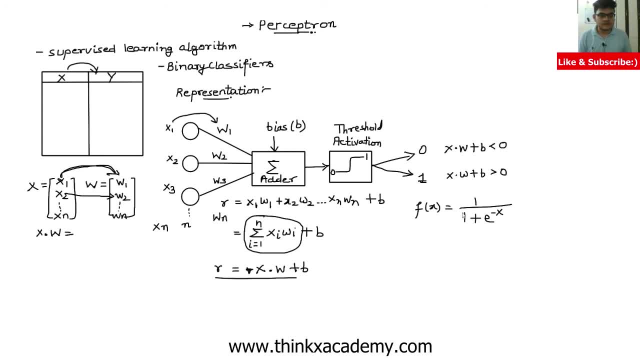 minus of x, right? So here, if we will give any real value of x, we will get a graph which was subtracted, Something like this. we have already studied this type of graph and we know that this is the value 1 and this is 0. so basically it can map this value to 0 or 1, which are basically two classes we can. 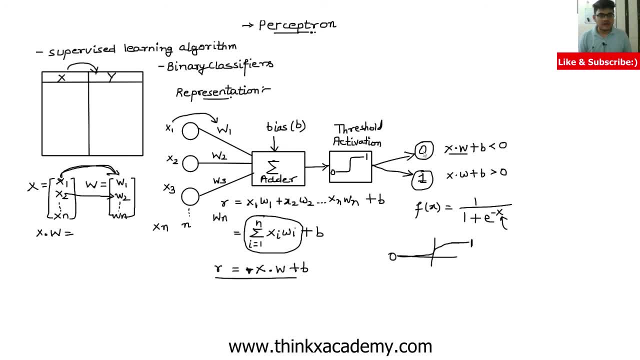 say that 0 represents that an email is a spam or not a spam, and similarly with 1 right. so it is basically classifying it into two different classes. So this is the basic calculations involved. now in the first there are iterations of this. 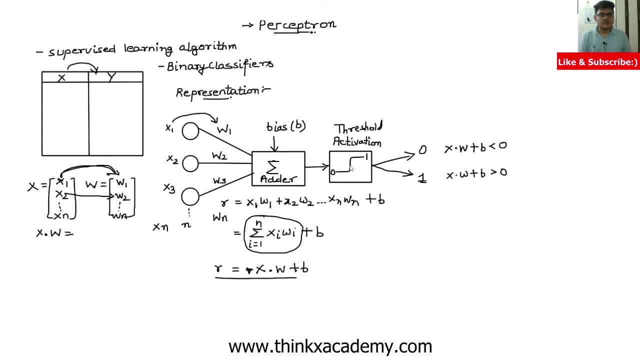 it. since it is a sigmoid function, it will give an output as 0 or a 1.. So it will classify it like this. So basically, a sigmoid function is this: f of x, 1 upon 1, plus e, raised to the power minus of x, right, So here. 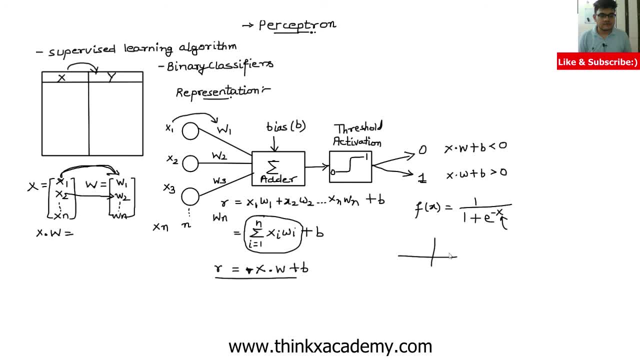 if we will give any real value of x, we will get a graph which was something like this. we have already studied this type of graph And we know that this is the value 1 and this is 0, So basically it can map this value to zero or one, which are basically two classes. 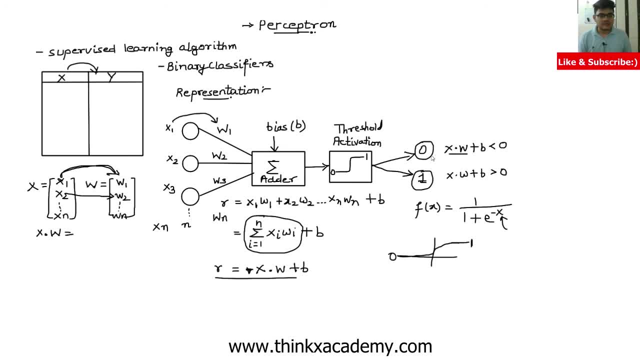 We can say that zero represents that an email is a spam or not a spam, and similarly with one Right. So it is basically classifying it into two different classes. So this is the basic calculations involved Now in the. there are iterations of this. 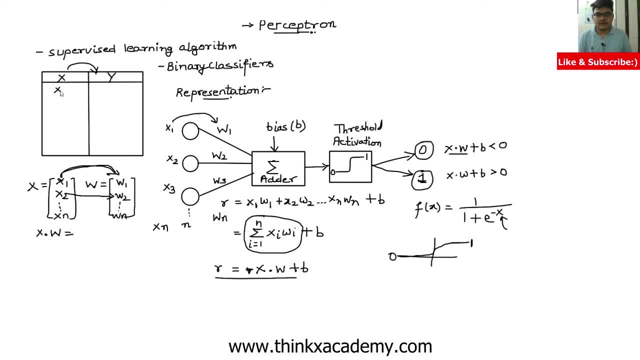 Right. So first we will take- let's say we take- the input here. I have some input and this input has some mapping here. Now what we will do is we will pass these inputs to this circuit. It will add them. We will choose some weights. Now, remember that these weights are adjustable weights. 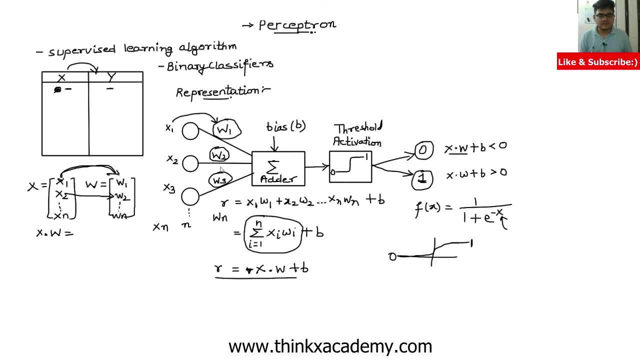 Right. So adjustable means that we can actually change them, and we will change them because we are getting some errors When, when we are calculating or matching it with the classes that we are getting Now. this means that if I will pass the input, the adder circuit will just give me this result and it will give the result to the activation function. 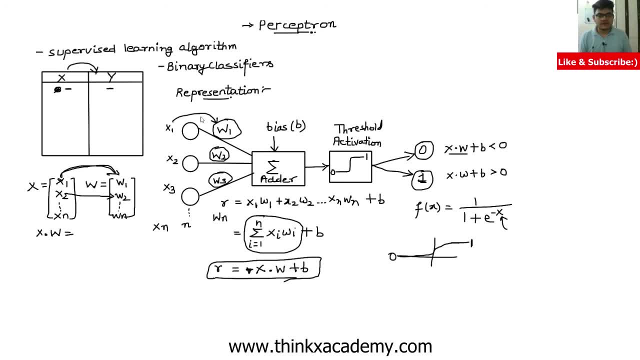 And let's say, after the first iteration and after calculating the first input, it classified it as zero. Suppose it classifies that as zero, But in the Y section it was mentioning that it is actually one. So in that case, what we will do is we will apply some learning rate. 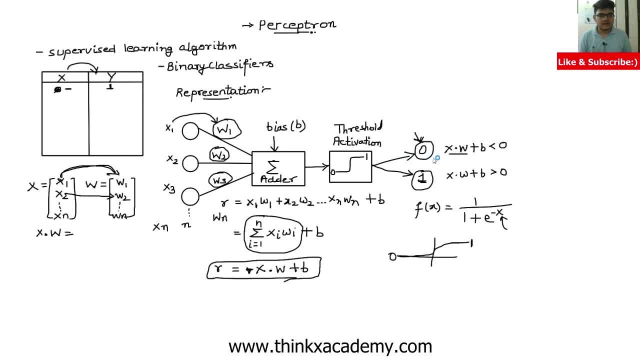 We will add some learning rate and we will calculate the error from here and we will adjust these weights according to that Right. So this will be W new Right. We will calculate the W new And the W old by adding some learning rate. alpha. 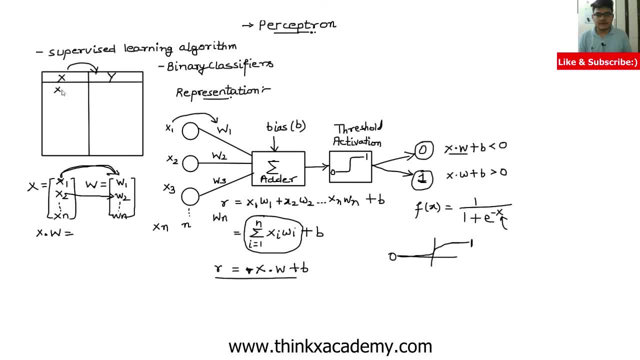 Right, so first we will take, let's say we take- the input here. I have some input and this input has some mapping here. now what we will do is we will pass these inputs to this circuit. it will add them. we will choose some weights. now remember that these weights are adjustable weights, right, so adjustable. 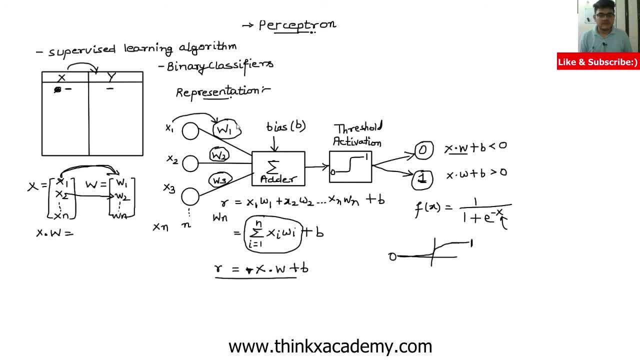 means that we can actually change them and we will change them because we are getting some errors when, when the we are carrying them, Calculating or matching it with the classes that we are getting now. this means that if I will pass the input, the adder circuit will just give me this result and it will give the result to the activation. 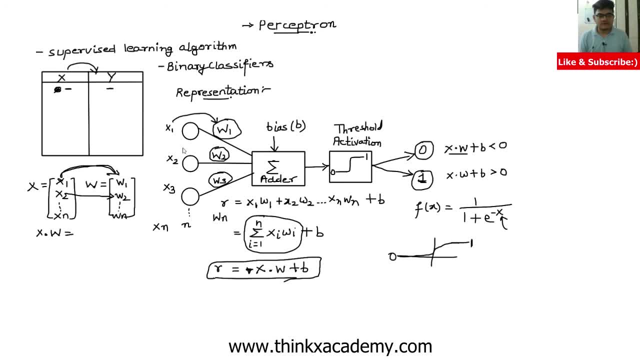 function and let's say, after the first iteration and after calculating the first input, it classified it as 0. suppose it classifies that as 0, but in the y section it was mentioning that it is actually 1. so in that case, what we will do? 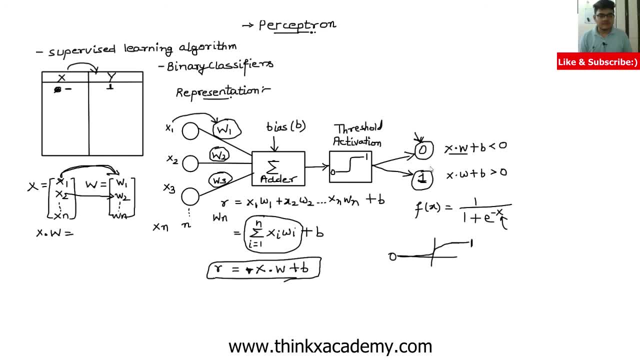 Is, we will apply some learning rate, we will add some learning rate and we will calculate the error from here and we will adjust these weights according to that right. so this will be w new right. we will calculate the w new and the w old by adding some learning rate, alpha, and we will also calculate the, the error that has. 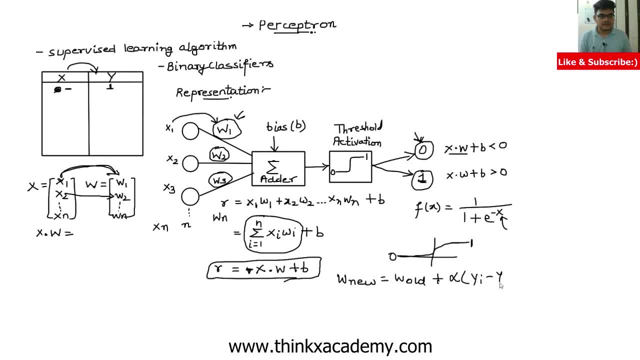 come here from y i minus y i bar. right, so we will basically just add the learning rate multiplied by this difference, which is actually the error. and here y i bar means the wrong output which we are getting from here, and y i means the right output, the output that is present inside of our data set. right, so we will calculate. then we will update the value of 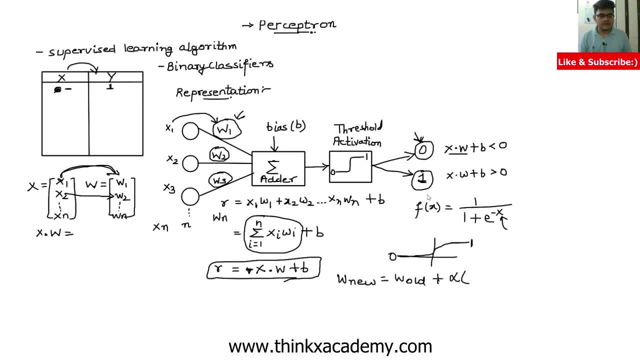 And we will also calculate the, the error that has come here from Y I minus Y I bar. Right, So we will basically just add the learning rate multiplied by this difference, which is actually the error, And here Y I bar means the wrong output which we are getting from here. 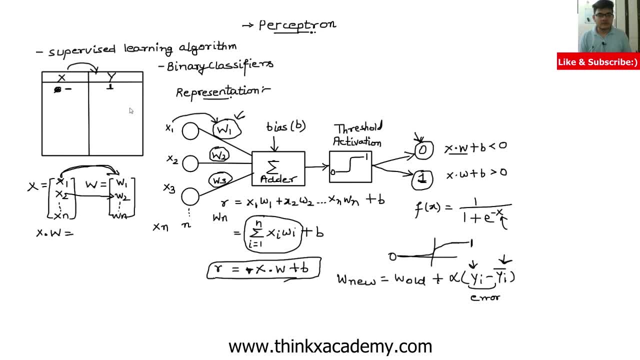 And Y I means the right output, the output that is present inside of our data set. Right, So we will calculate, then we will update the value of The weights here and similarly in the Next iteration when we will update these ways, then these weights, then we will again calculate the result. 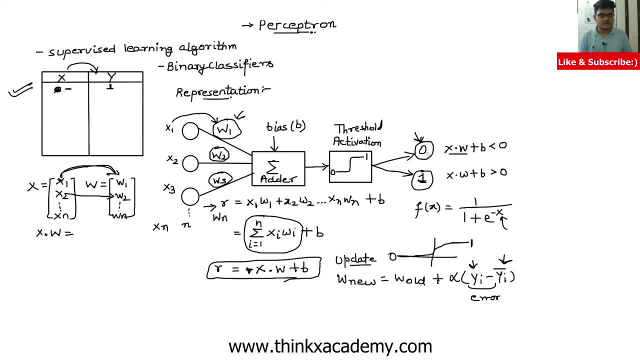 and again we will pass it to a threshold function and again we will get some output here And we will then tally it with the table, with the data set or the table we already have here, And again we will calculate the error, multiply it with some learning rate and basically learning rate should be chosen wisely. 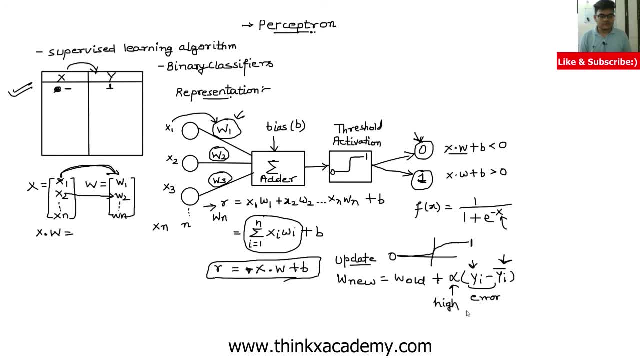 because if the learning rate is too much, it is going to do overshooting of some values. We have already studied this in the gradient descent video- and if this learning rate is very low, it will take a lot of time and there are some trade offs of choosing the learning rates. These are the trade offs, right, So we will multiply it with. 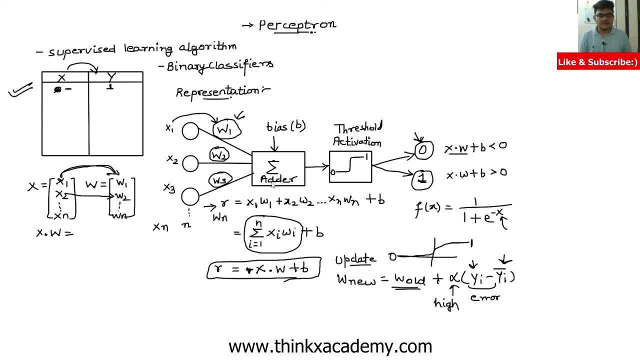 the error and we will add it to the old weights and, similarly, we will do this again and again until and unless we will get the right output, which means that the error will come out to be 0, and after this, the perceptron will get trained, the learning algorithm which is the perceptron. 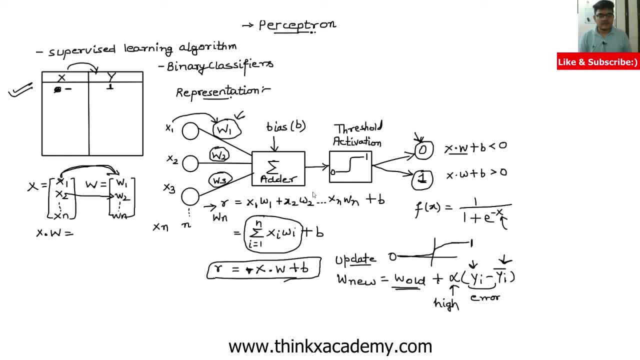 learning algorithm. It will get trained and, similarly, we will be able to do the classification, the binary classification. So in the next tutorial we will solve an example. we will solve an example where I will I will do the classification of the learning algorithm and I will do the classification of the 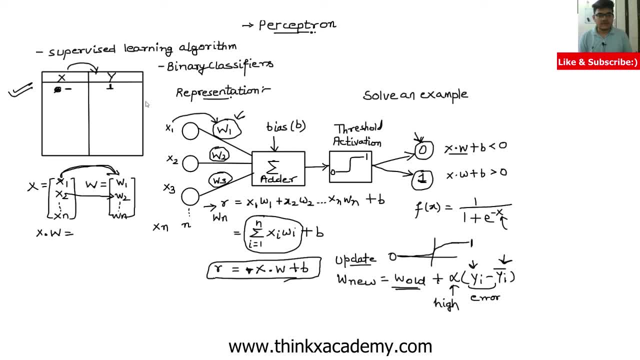 learning algorithm. Give a very simple data set and we will see how we can actually perform these operations and we will see how we can train the perceptron to adjust or to converge to the solution. So in the next tutorial we will do that. So that's all for this tutorial. If you have,